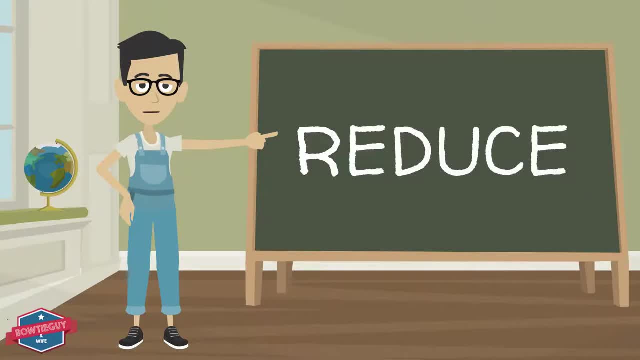 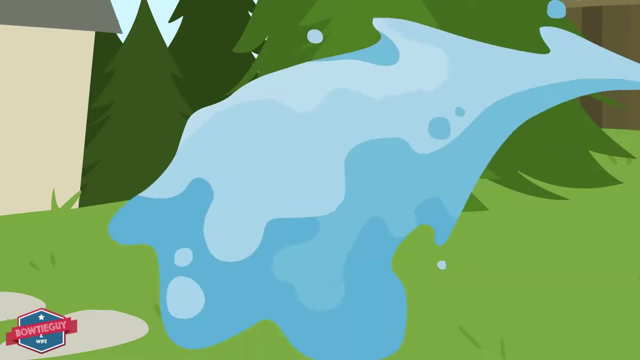 Let's become a conservationist. There's three words that you need to know. First, let's talk about reduce. To reduce is to cut down on the amount of resources that are used. So, in thinking about conservation, how can we reduce the amount of resources that are used? Well, if you're a 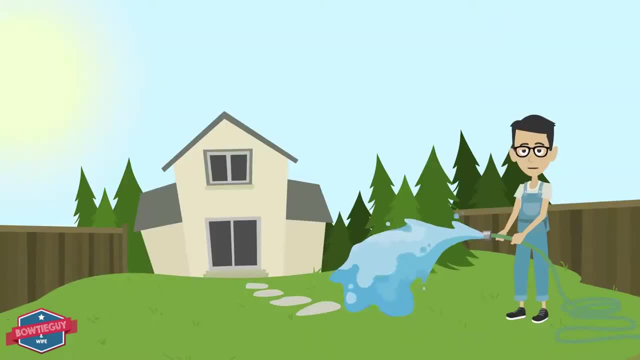 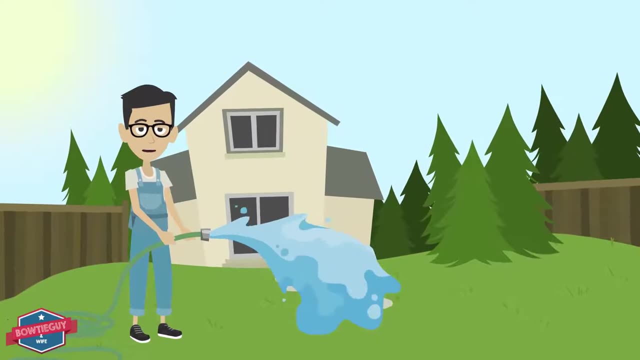 conservationist, you should reduce the amount of water that we use to water our lawn. So if it's summertime, don't water in the heat of the day, So around noon, don't even think about it. You should water in the early morning or the late evening so that the water can seep into the soil. 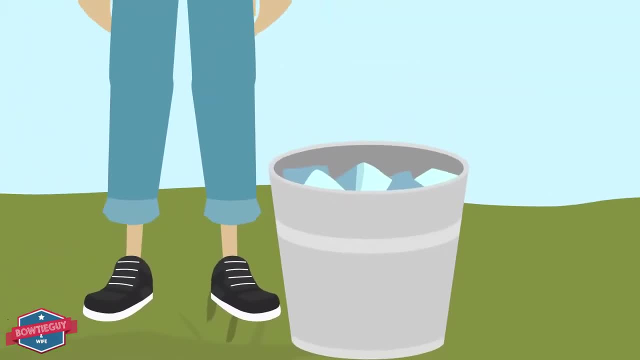 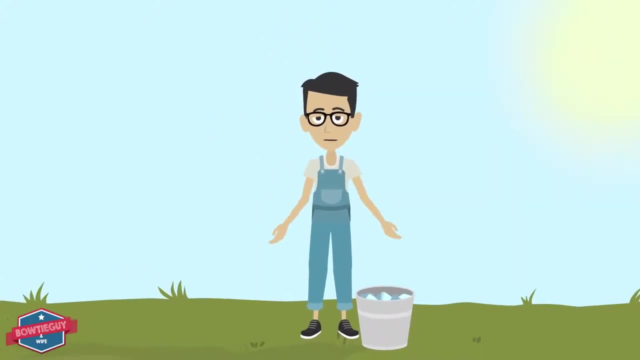 and better hydrate the roots. I can't help but to think back to my experiences around the world, looking at the men and the women and the children, and how they desperately just wanted a sip of fresh water. How could I be so wasteful? We need to reduce the amount of water that we're 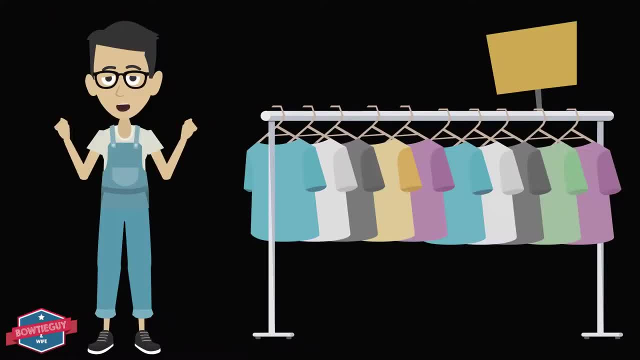 wasting. We need to reduce the amount of water that we're wasting. So if it's summertime, the next time you're perusing through your closet, take a look at the inventory of clothes that you have. Do you have too many? Do you have some that are too small? Perhaps, maybe a brother. 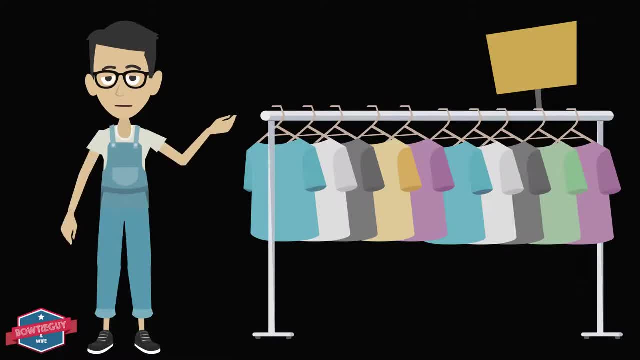 or a sister could benefit from you giving some shirts or pants to them, Or you can donate to your local thrift store, where surely someone could benefit from the use of them. The average American family could greatly reduce the amount of electricity that they use throughout the day. 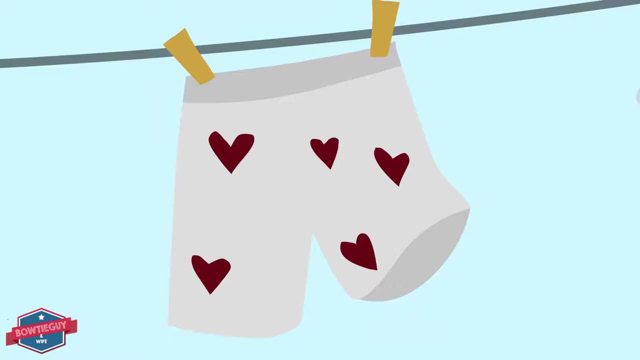 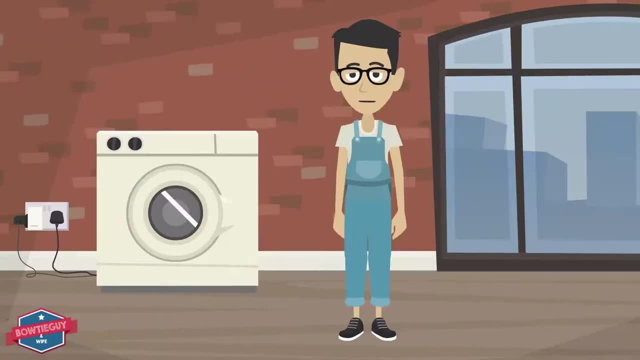 Do you have a dryer? Did you know that you can also dry clothes using the sun's energy? Using a dryer uses a lot of energy that could possibly be conserved or reduced When traveling very short distances instead of using a car. perhaps, maybe you could. 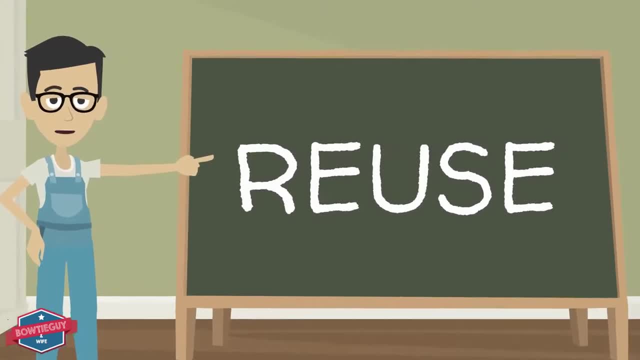 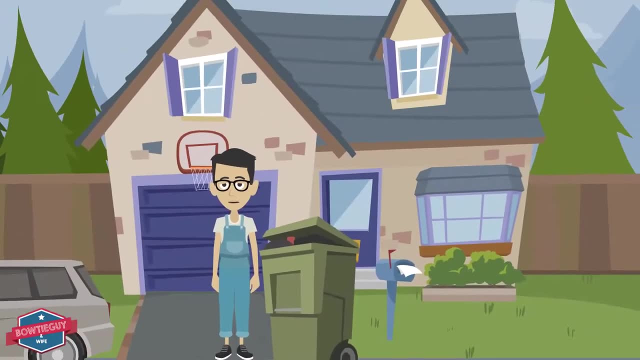 walk. Hmm, what does it mean to reuse? To reuse means to not throw away things that could be used again. I know it may sound disgusting, but some of the things that we throw away probably shouldn't be thrown away. We could use them again and again for different purposes. 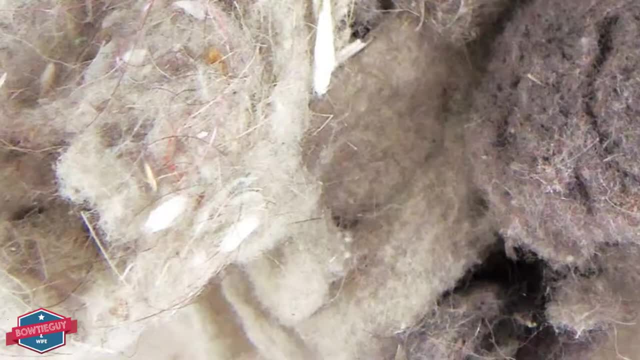 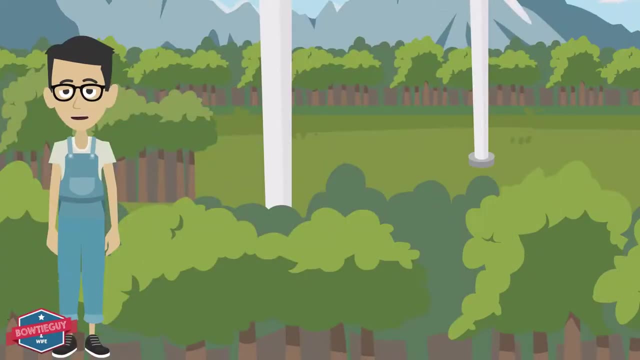 Throw away lint from the dryer? I think not. Lint is an excellent fire starter that you can use in your fireplace. All this talk about reusing makes me think about renewable energy sources. Take a look at these wind turbines. The wind is constantly. 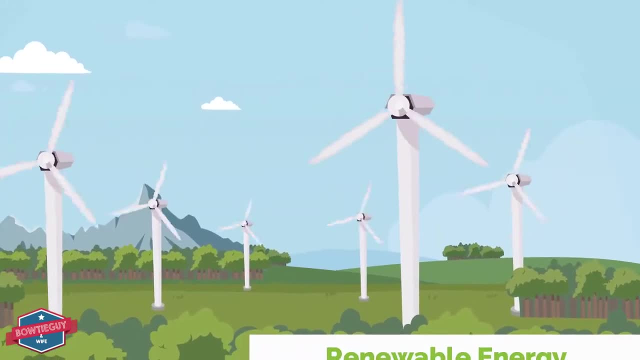 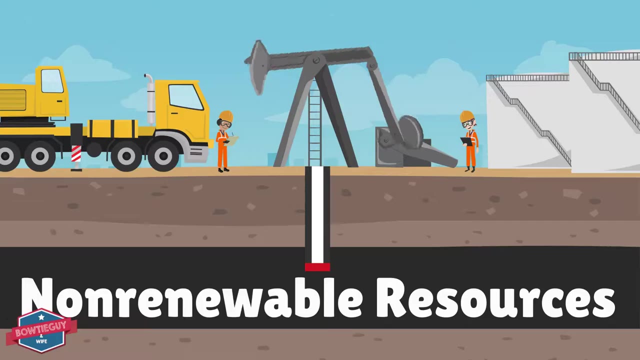 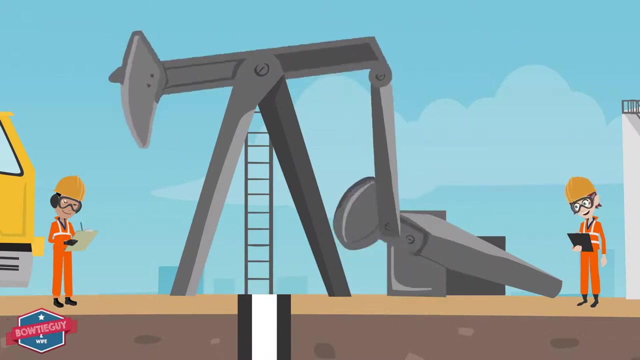 blowing and water all over earth is constantly flowing. So think about it. Those renewable energy sources can be used to generate electricity. Unfortunately, many people around the earth utilize non-renewable resources. Non-renewable resources include coal, gas and oil. They're. 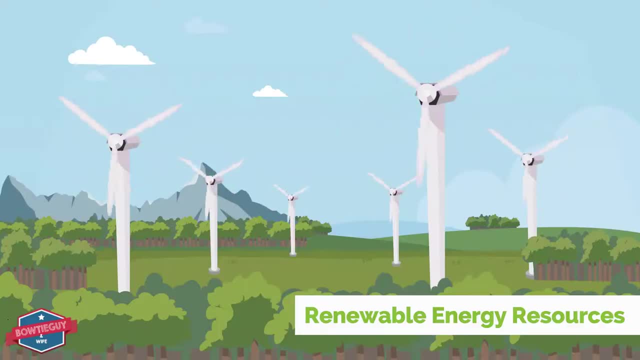 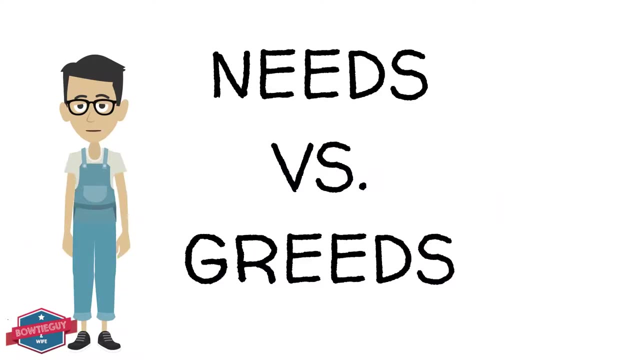 not going to be around forever, so we have to utilize renewable energy resources such as wind and water. When thinking about reusing, think about your needs versus your greens. Do you really need that new item or could you do without it? If you really want to put forth the effort and 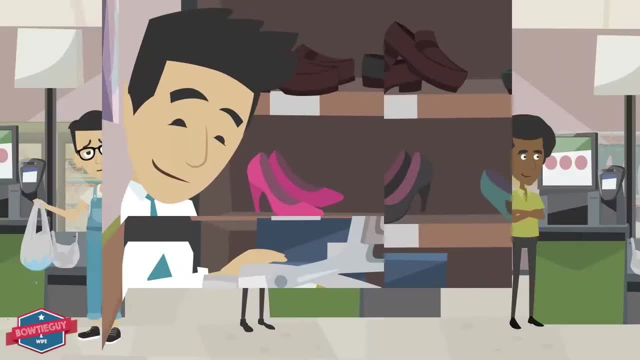 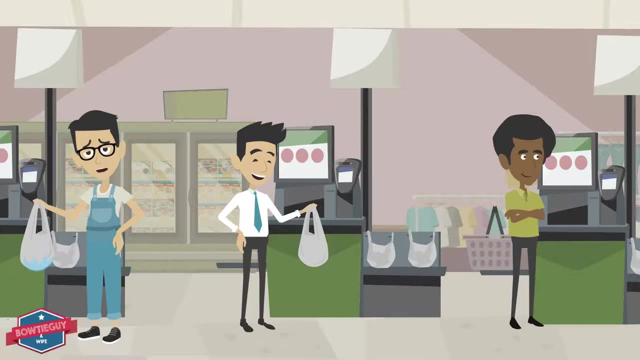 think about it. there are plenty of things that we could reuse. Many grocery stores utilize plastic bags. Plastic bags are bad for the environment, so why not bring a bag that we can reuse over and over again? A cloth bag is a great example. Single-serve plastic water bottles are not. 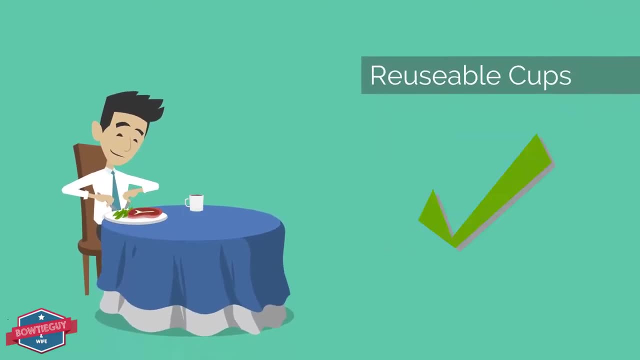 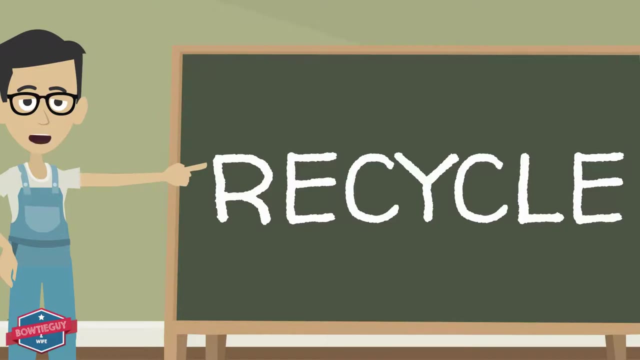 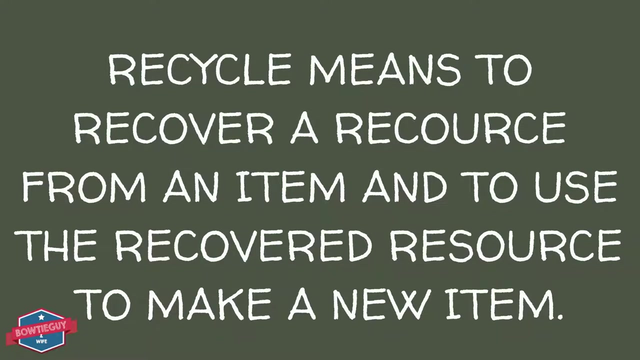 good for the environment and they may not be good for your health, so why not use a refillable, reusable container for your needs? What does it mean to recycle? To recycle means to recover a resource from an item and to use the recovered resource to make a new item. 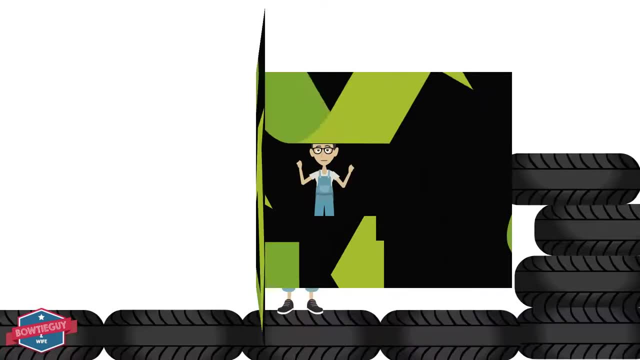 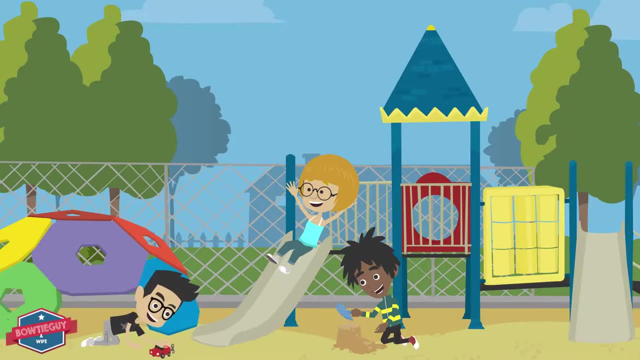 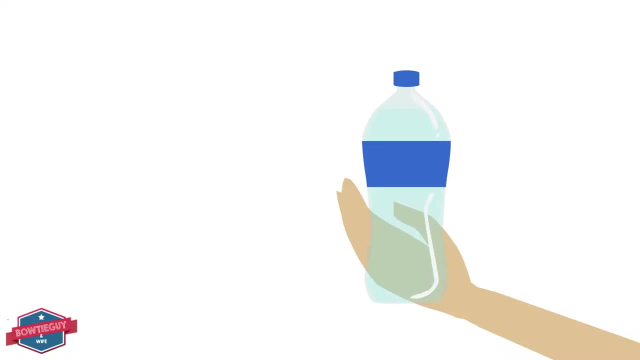 This is the Universal Recycling System. It's a universal sign for recycling. What happens to tires when they're all used up? Well, some people actually recycle tires into mulch for playgrounds. Where do plastic water bottles go after they're used? Did you know that some companies can actually convert the 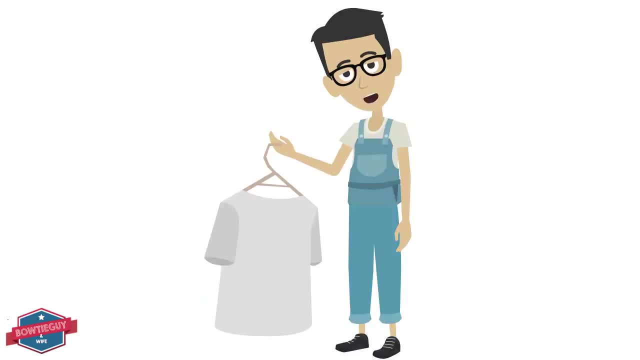 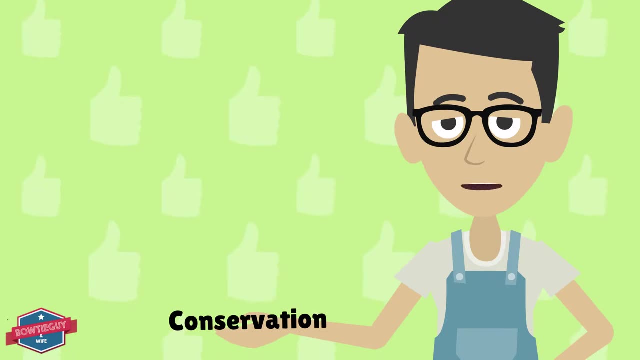 plastic from the plastic water bottles into clothing. Yes, it's true, Conservation doesn't have to be difficult. We need to conserve Earth's resources. To To better conserve Earth's resources, we need to learn to reduce, reuse and recycle. 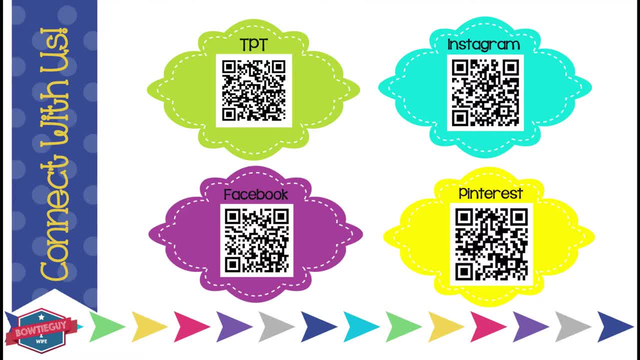 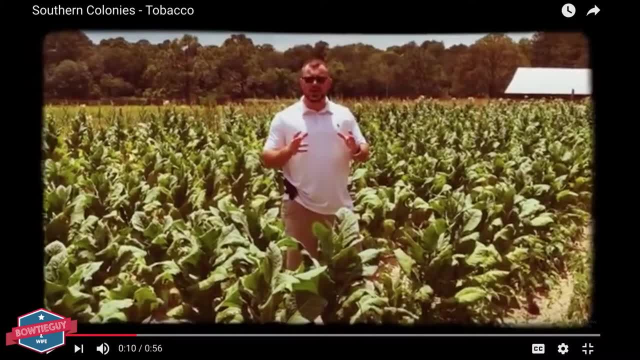 Thanks so much for watching. Feel free to check out our Teachers Pay Teacher Store, Follow us on Instagram, like us on Facebook and check out our Pinterest boards. Feel free to check out our YouTube channel, where you can check out many exciting videos like the one that you've just seen. 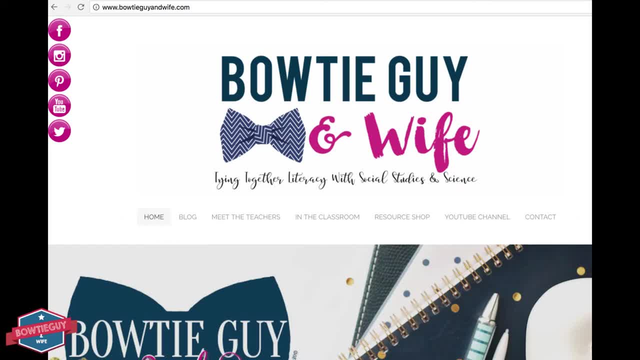 And head on over to our blog at wwwbowtieguyandwifecom. See ya.